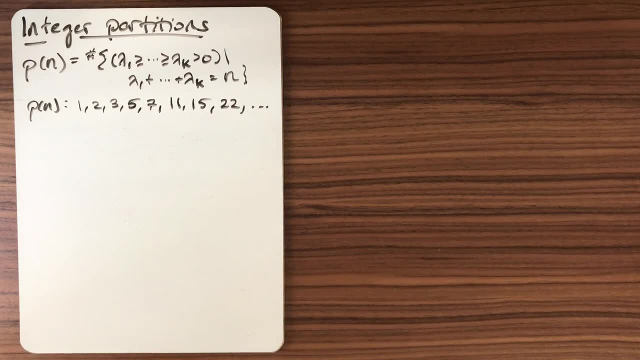 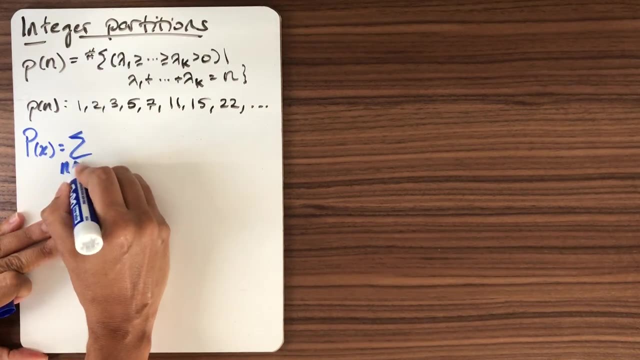 and we saw that what we talked about. there's no closed form for this. however, we did find a closed form for the generating function, capital p of x, which the definition is the sum n greater than equal to 0, of p of n, x to the n, and the formula we derived last time is: this is going to be an: 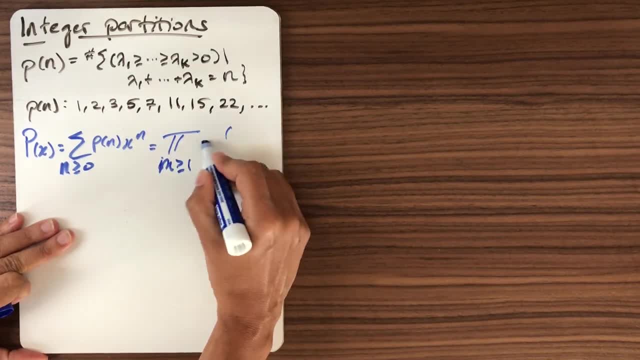 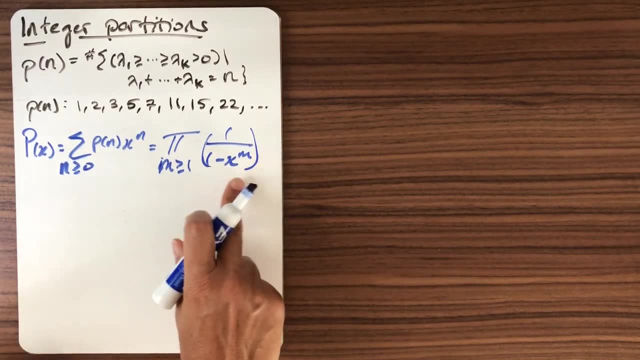 infinite product, Say of m greater than equal to 1, 1 over 1 minus x to the m, and our combinatorial interpretation of this is important. Here we're thinking of 1 over 1 minus x to the m, Choosing a term out of this. 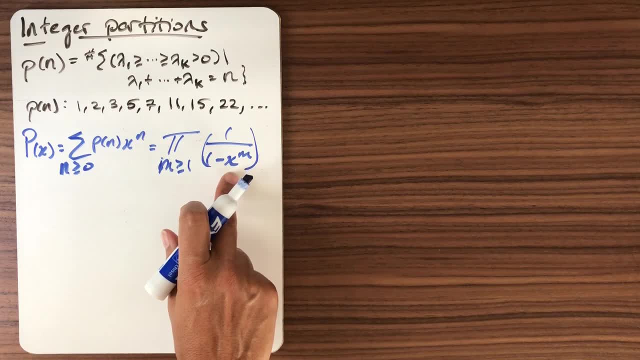 infinite sequence is the same thing as choosing how many parts are equal to m. So we're going to keep that in mind and we're going to think about a refined way to understand these integer partitions. and the way we're going to come about that is by looking at a two parameter. 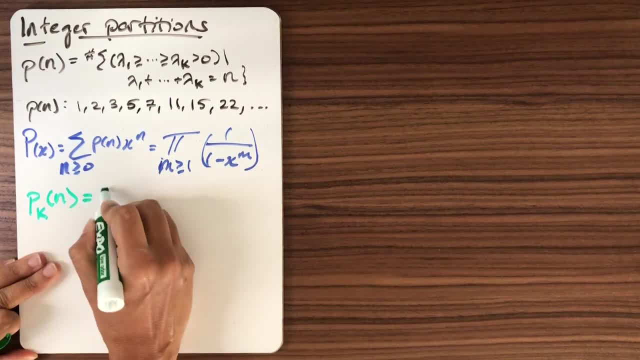 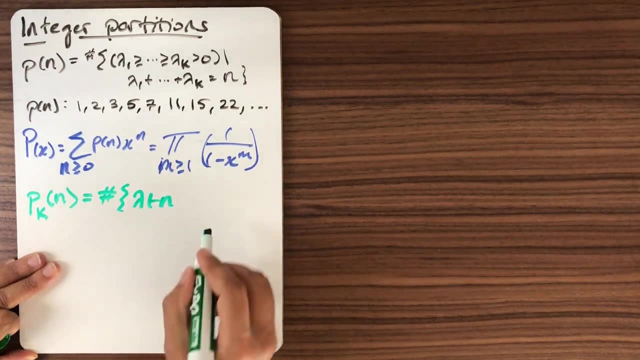 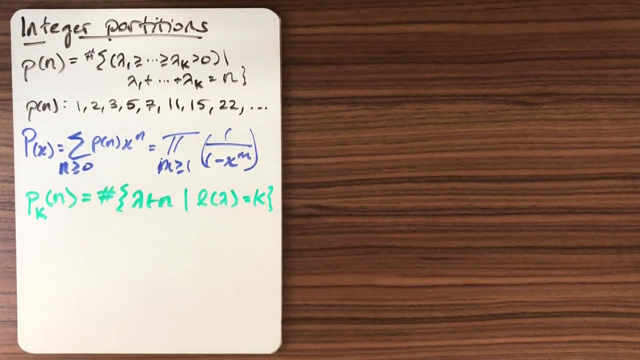 count P of n, k, and this is going to be the number of integer partitions of n, which we can denote with this notation, such that the length of lambda, the number of parts, is exactly equal to k. This is a refined way to count the number of integer partitions. So if we were going to count for 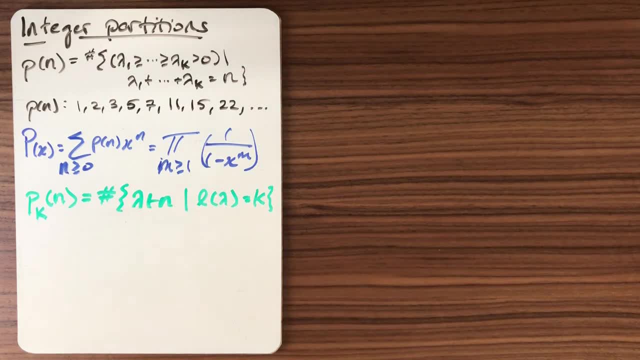 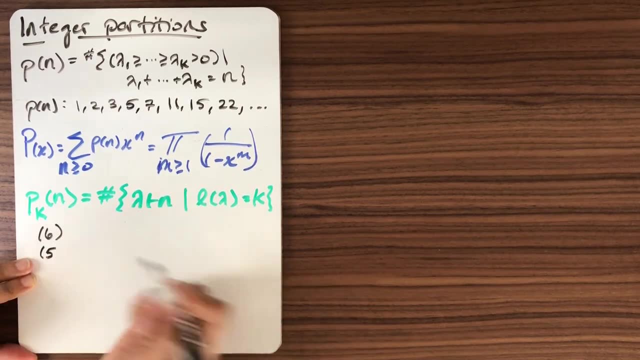 example, the number of integer partitions of 6.. If we were going to enumerate them, there are 11 of these. We could do them lexicographically, so always start with the biggest number of integer partitions. So this is the biggest number you can, 5 is the biggest number, and then 1.. We could do a 4 and a 2.. 4, 1, 1.. 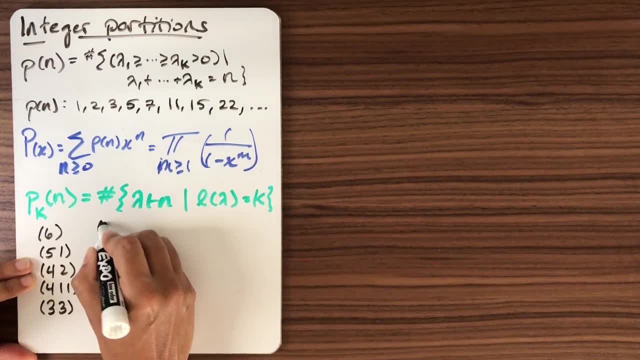 We could do a 3 and a 3.. We could do 3, 2 and then 1 left over, or we could do 3, 1, 1, 1.. When we start with a 2, we want to take the biggest number possible next. 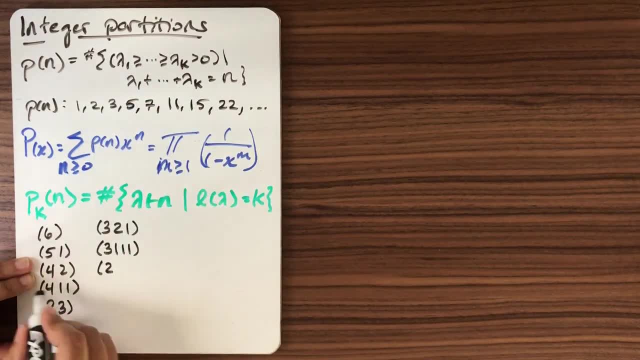 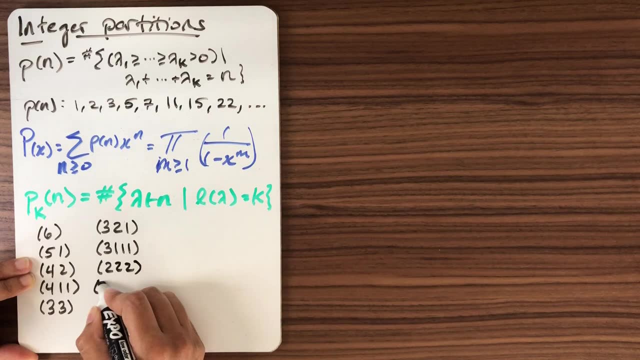 Now we can't take a 4, because we need to write these in weakly decreasing order, and we've already written 4- 2.. So there's no point writing 2- 4. So the next biggest number is 2.. So this is really the imperative. 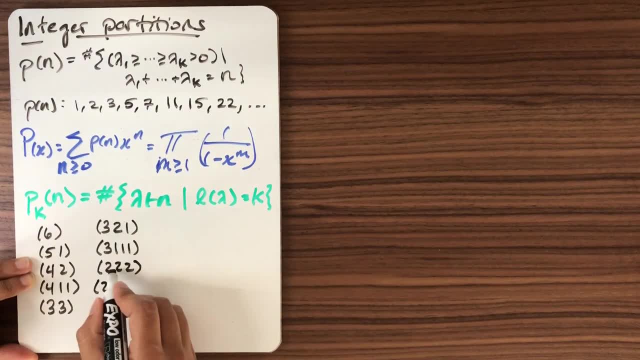 To get in a nice recurrence for the number of partitions of N is this idea that we kind of have to were restricted on what comes next by what came before. So we could do it this way: We could do 2: 1, 1, 1, 1, or we could do 1, 2, 3, 4, 5, 6.. 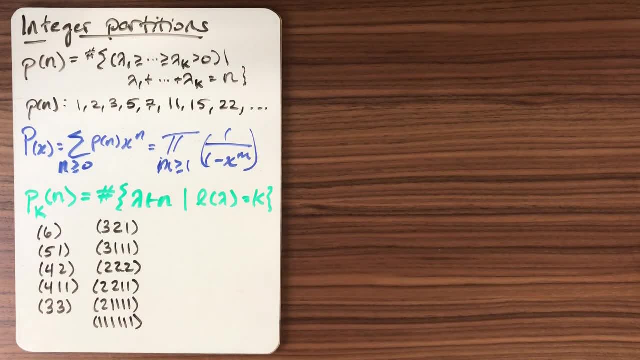 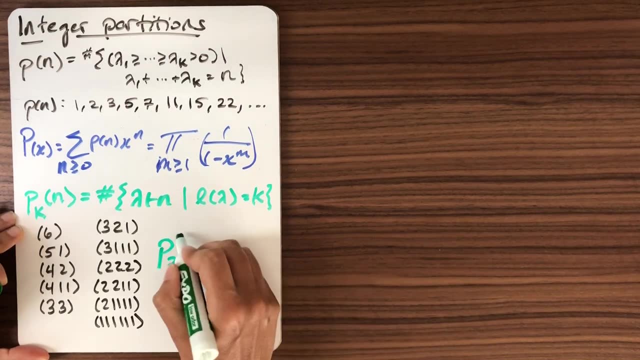 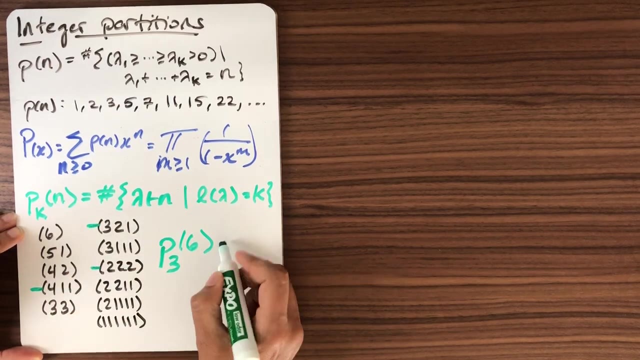 Now, if we want to take this number, pk, in, and we want to say, OK, well, there are 11 integer partitions of 6, and we want to say how many of those have exactly three parts, then what we could do is just sort of check off our list: this one does, this one does, and this one does, and we 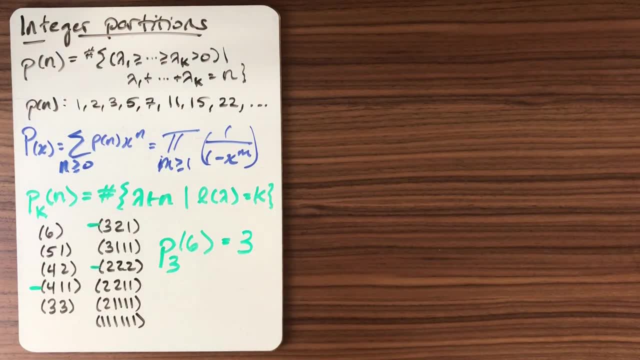 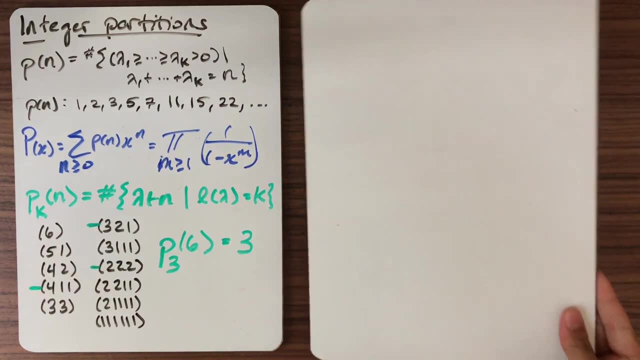 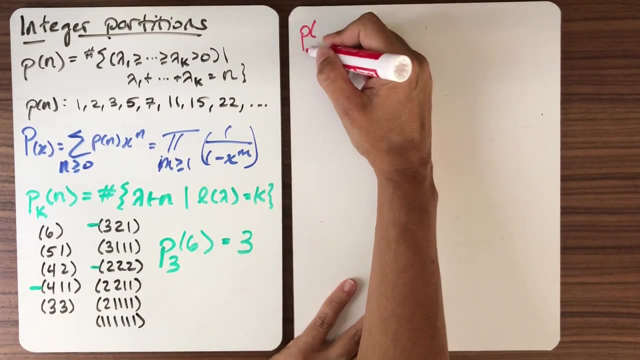 find this number is equal to three and what we want to do is think: okay, well, systematically, is there some way that we can think about these numbers? and the recurrence relation that we talked about in discussion that we came up with is a lovely recurrence: P K of n is equal to P. well, we can think about these things. 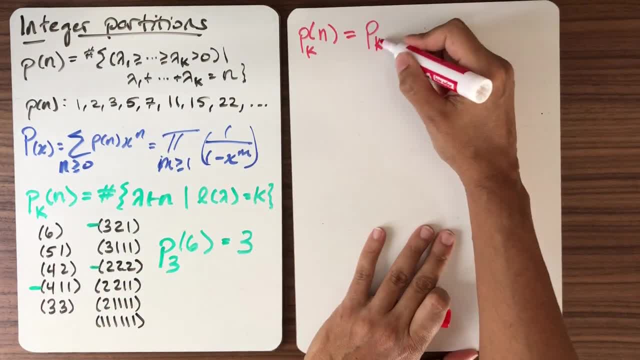 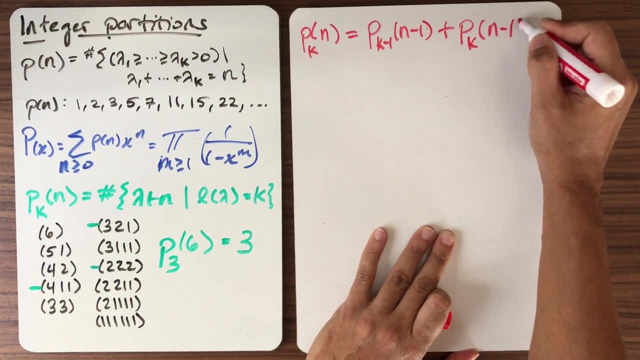 either your last part is equal to one, in which case you can just take that part away, or your last part is not one, in which case you can take one away from every part. so let me write down what this is. the combinatorial proof is this: 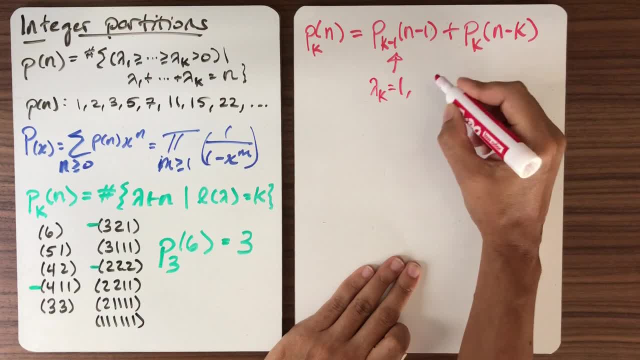 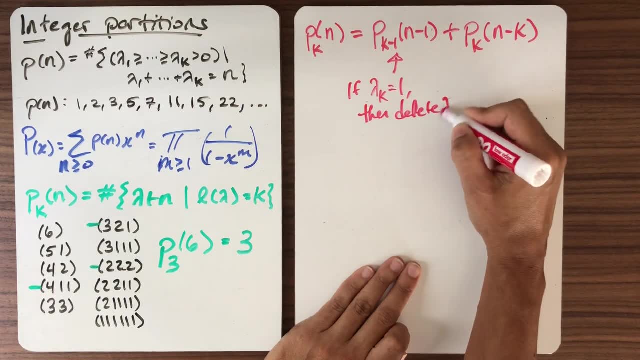 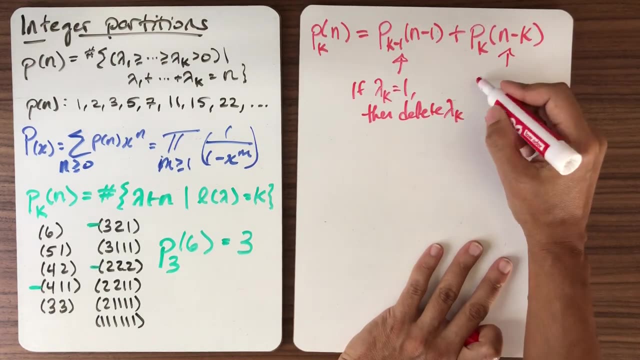 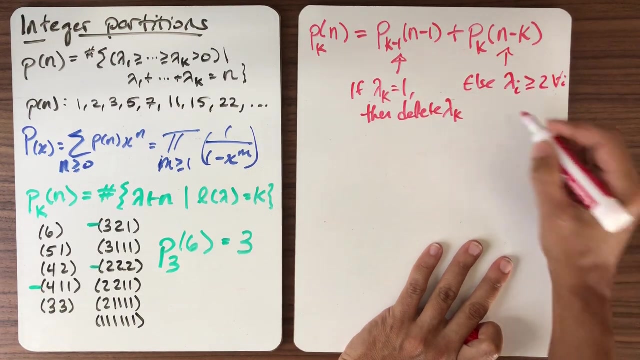 is if lambda K equals one, then delete it. so we've lost one from n and one part, and this needs to be the otherwise case. so else in this case, lambda I is greater than equal to two for all I, and so what we're gonna do is: 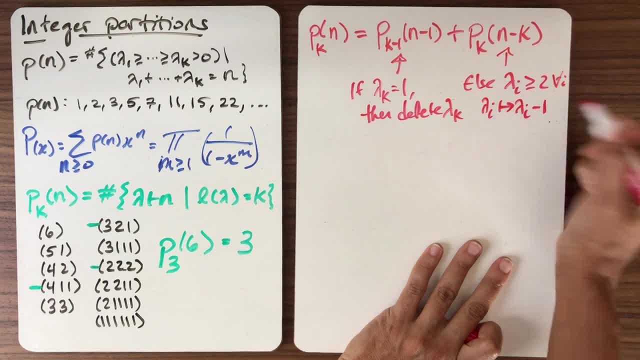 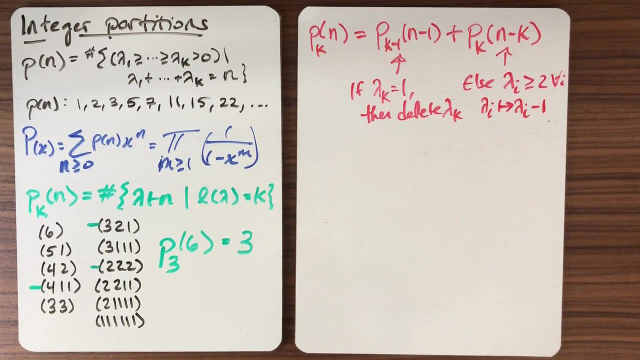 we're gonna replace lambda I with lambda I minus one. that's gonna give us an integer partition of n minus K, because there are K parts from which we lose one each and we still have K parts remaining. so that's our combinatorial proof of this recurrence relation. that allows us to think about this recurrence relation. 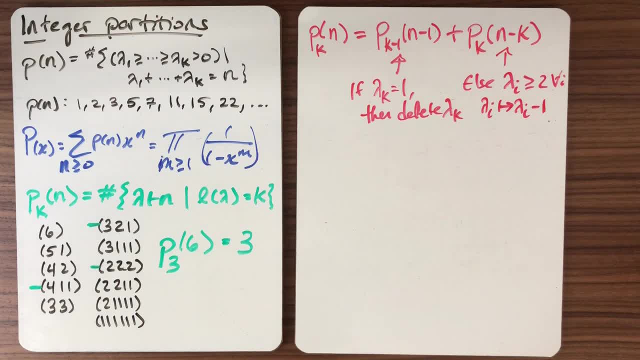 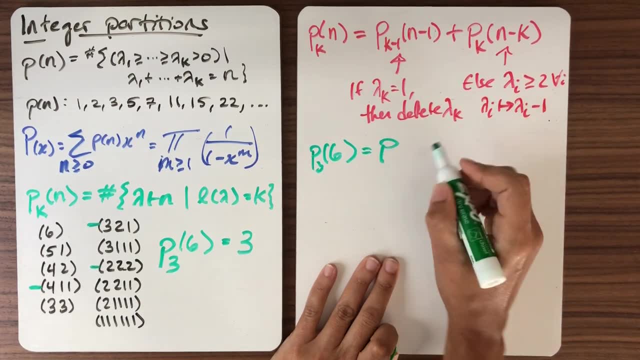 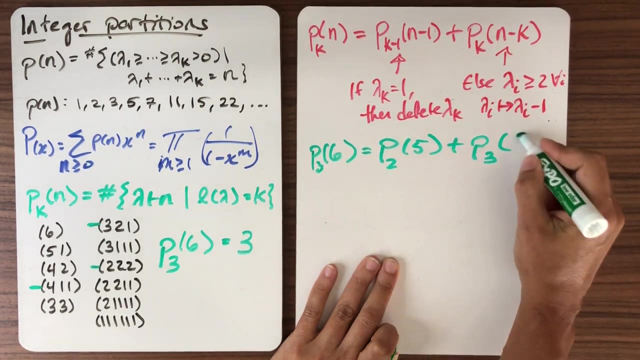 so it allows us to compute these numbers fairly quickly, and if we look at this example, we can see that P three of six is equal to P two of five, plus P three of well, six is three. so when we write down the elements that we had here, the 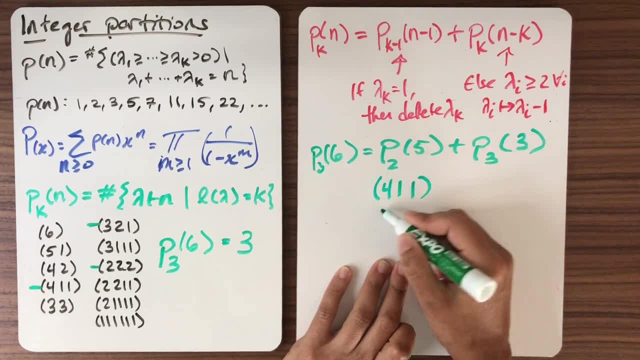 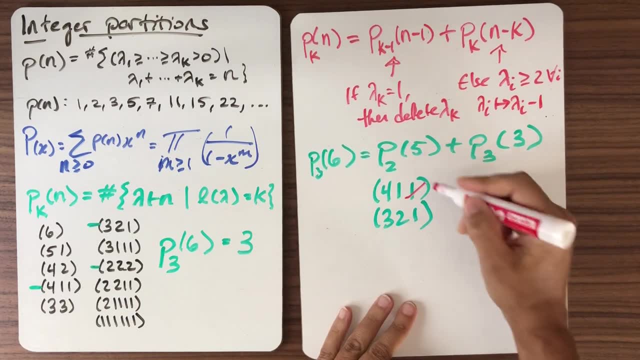 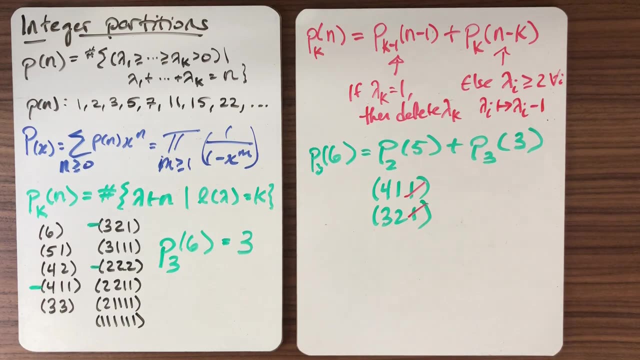 parts that ended in one. we had four, one one, and we had three, two, one, and we can see that, yes, taking these last parts away, deleting that and deleting that gives us an integer partition of 5, with two parts and taking one away. so the 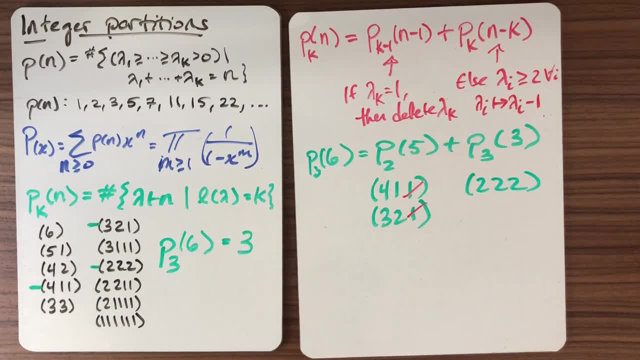 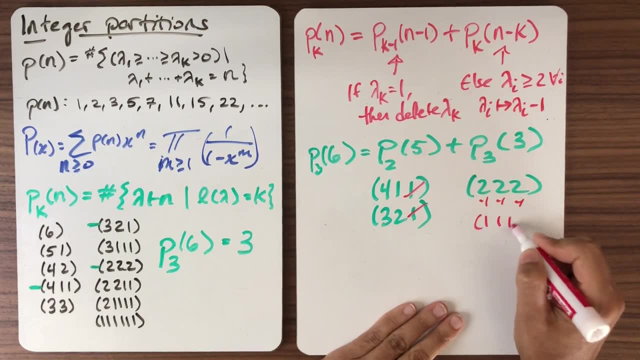 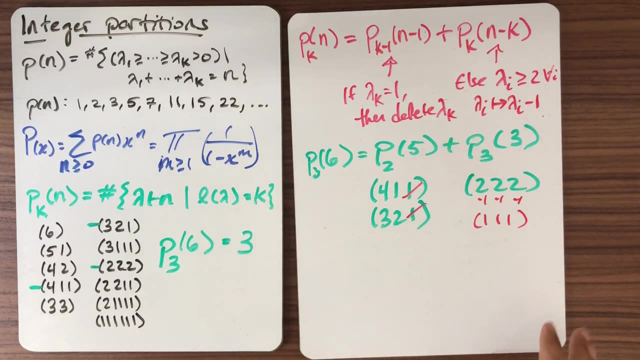 other thing that we had was 2, 2, 2, and we want to get end up with partitions of 3 into 3 parts, and of course there's one way to do this, which is just getting this partition. so that's a way that we can understand these pkn's. and now we 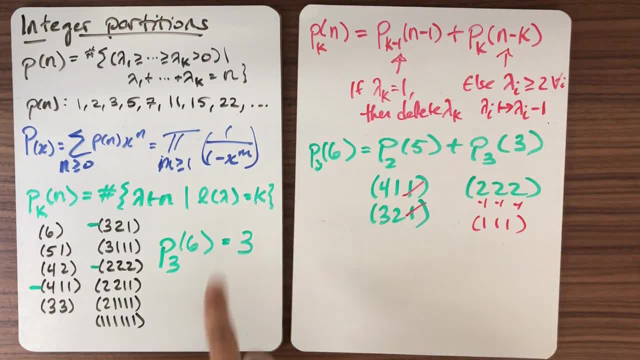 say, well, can we get a generating function for these? so these have this nice recurrence. how does that really work here? here we're not interested in the number of partitions, but the size of the partition, and we want to ask ourselves: is that really different? so the answer is actually not at all. if we 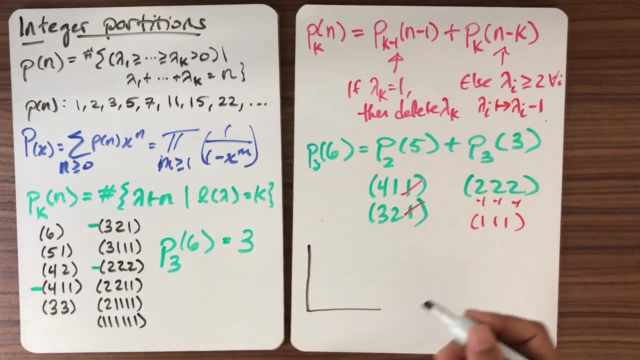 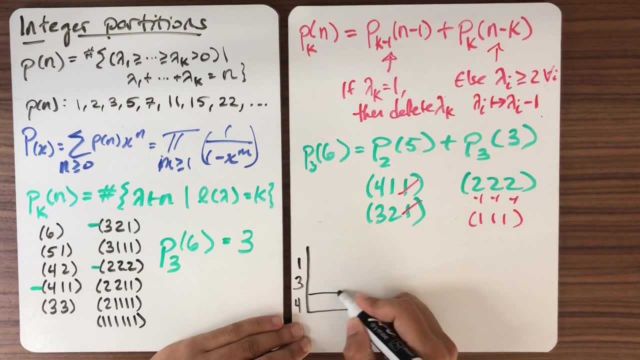 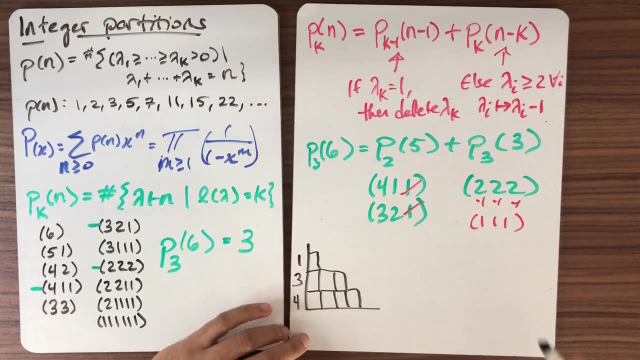 think about drawing the integer partition. so if we take a partition, for example, let's take something like 4, 3, 1, I can think of drawing this with boxes in a row, similar to our Lego construction that we had- or 3, 1.. So this is a way to 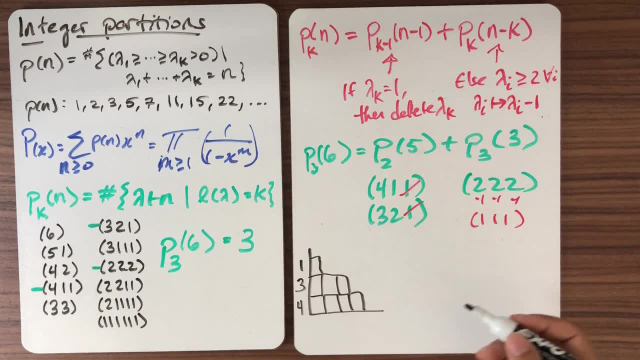 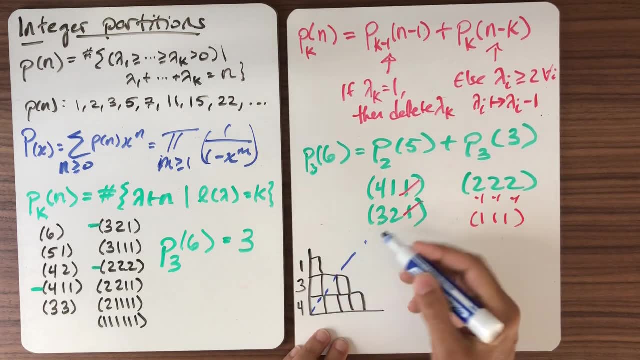 graphically represent the partition 4, 3, 1. and once we have this paradigm, we can think about things we can do to this picture. one obvious thing we can do is we can look at the main diagonal and we can reflect it, reflect the diagram. across the main diagonal. when we do that, we can also have to look at the other intersection, because we still have these elements right in front of us. if we do that, it makes sense right, because we build up a sqrt�uld and the возération is. 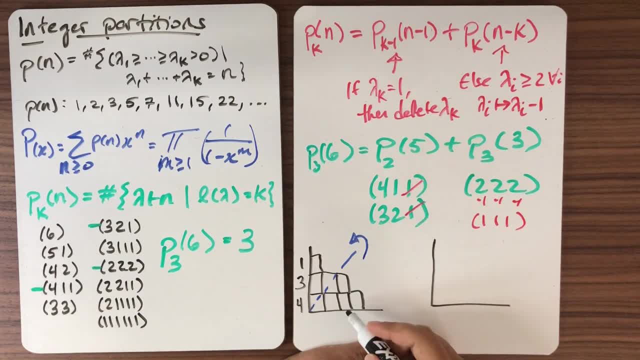 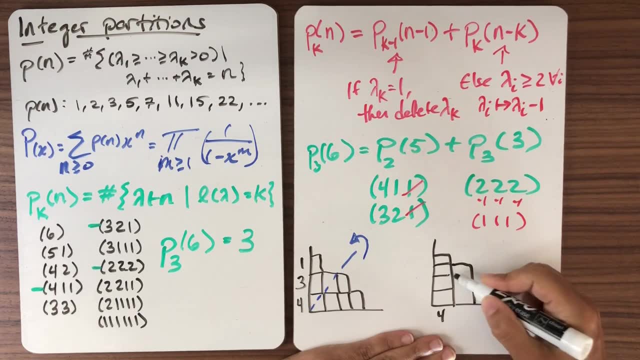 that what is the integer partition that we end up with? well, here this is going to go vertically: one, two, three. so this is going to be the four is going to be the height. three will be the height of this one and one will be the height of. 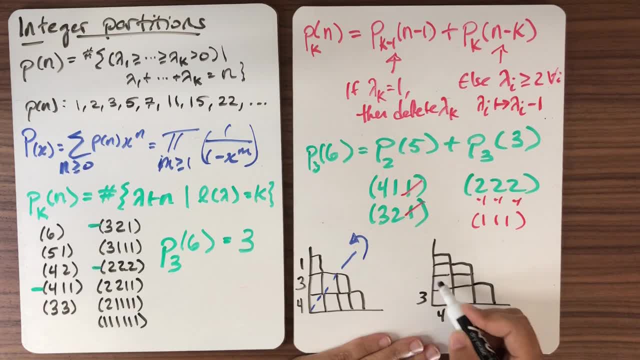 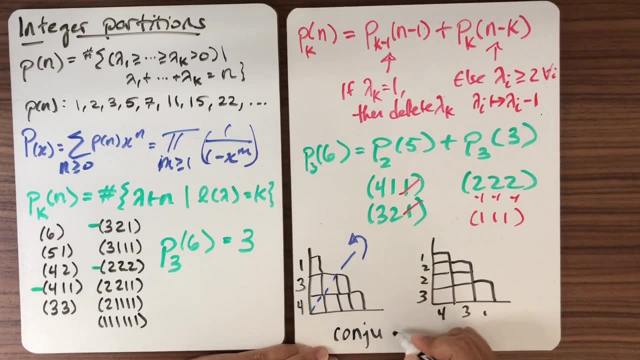 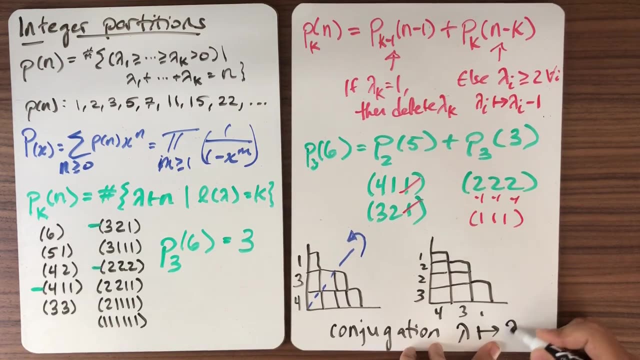 this one. but now, if we read the rows of it, we get a different partition: three, two, two, one, and this is what we know as conjugation. so this is the conjugate of an integer partition. if we start with lambda, the conjugation is often denoted. 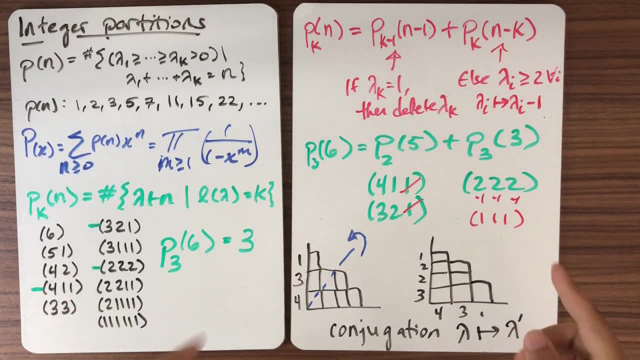 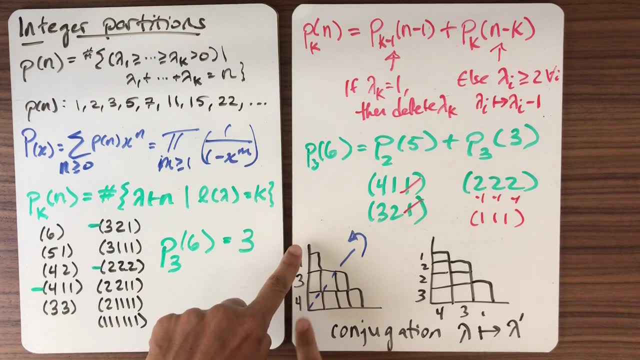 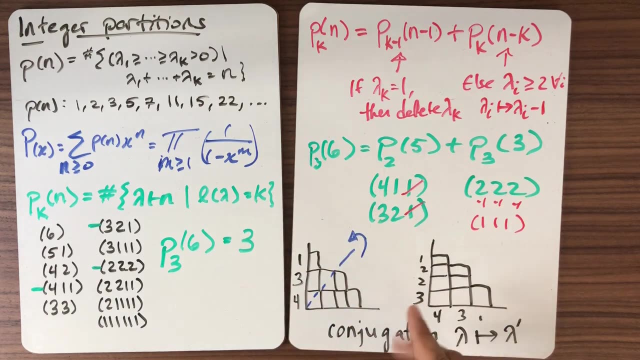 with a prime, and now we can think about this. partition into K parts has a nice graphical interpretation in this paradigm. here I have a partition into three parts, right, because that's giving me the height. what happens when I do this? transpose the height that I have here, which tells me that I have three parts. 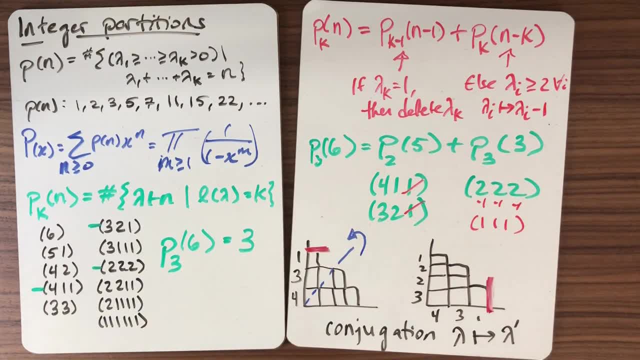 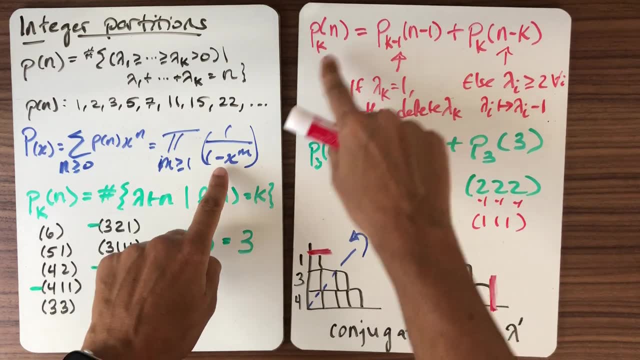 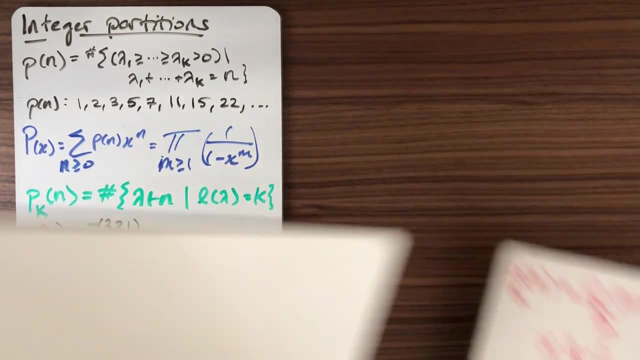 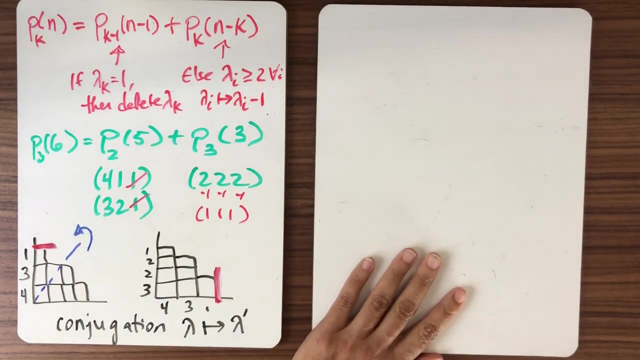 becomes the size of the integer partition, and so that's what's going to allow us to make a relationship between this amount, this PKN, and this generating function. so maybe we'll keep this board. so remember that we had this generating function for all partitions of n, which 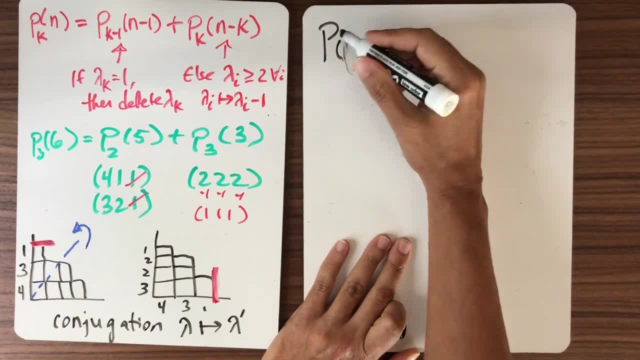 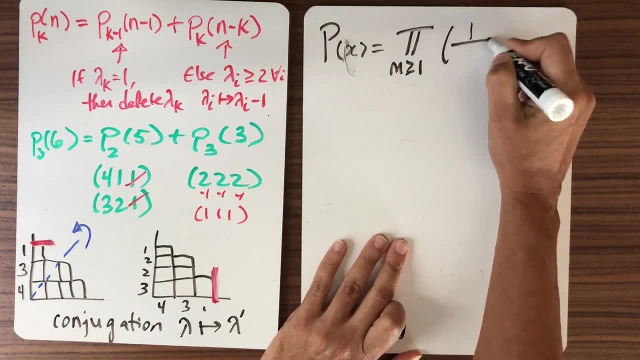 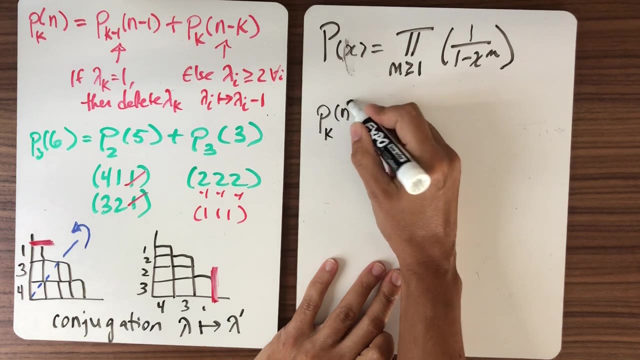 is P of. excuse me, X is equal to the product of M greater than equal to 1, 1 over 1 minus X to the M. and now this PKN we want to think about. can we get a generating function for that? well, this one. we have this recurrence relationship, but here we. 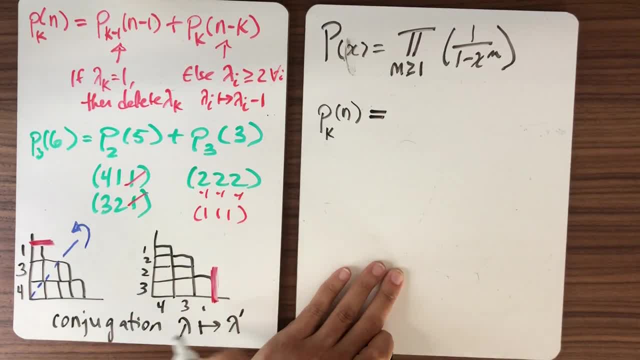 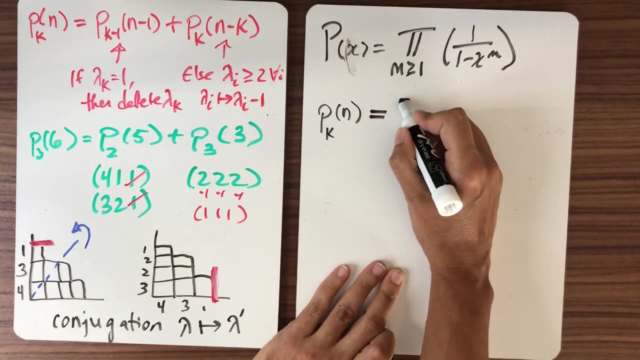 can think of these in a different way. by this bijection of conjugation. it's an involution, right? so it's a. it's a bijection on partitions and it changes this condition of K parts to: the biggest part is equal to K, so this is the set. this is, by definition, that cardinality of the. 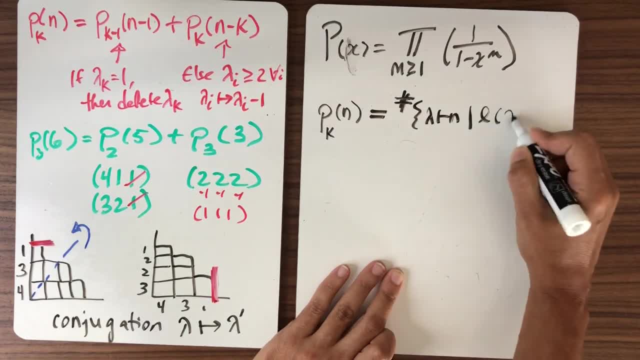 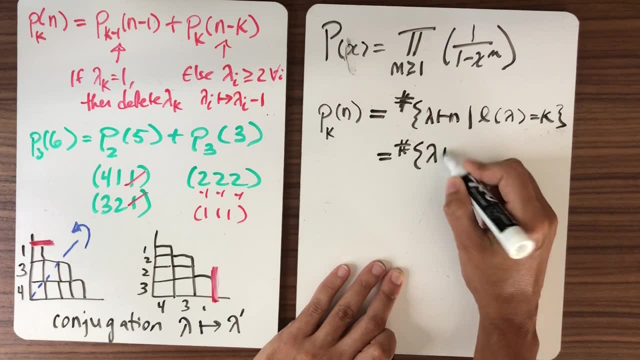 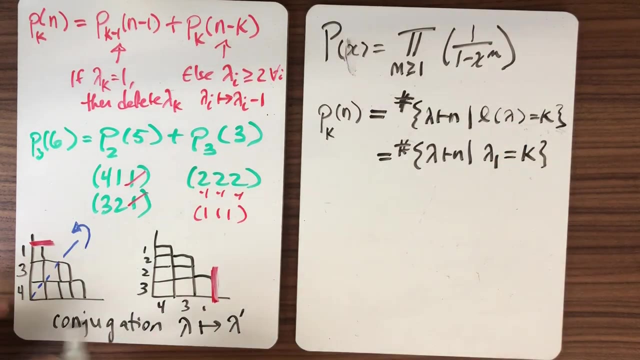 set of lambda is a partition of n, such that the length of lambda is equal to K, and this is in bijection with the number of partitions lambda of n, such that lambda 1 is equal to K, and this relationship between the length, which is the height in this picture, and the size of the largest part. 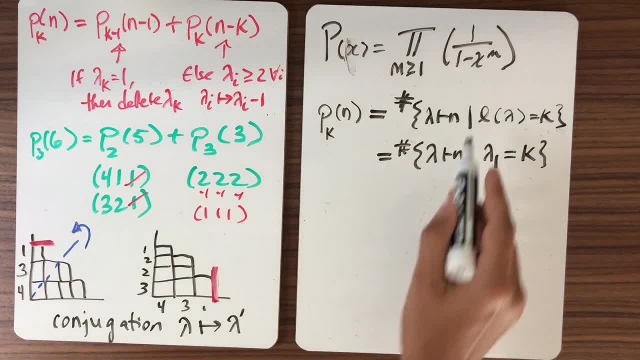 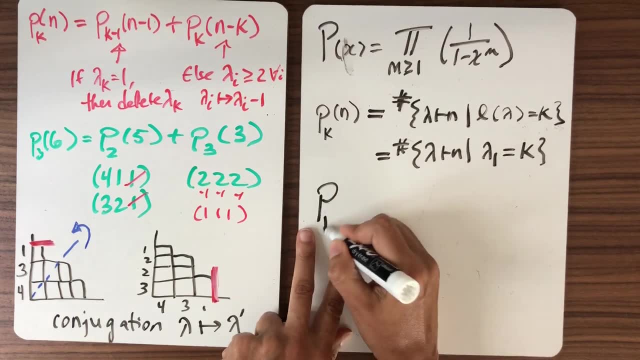 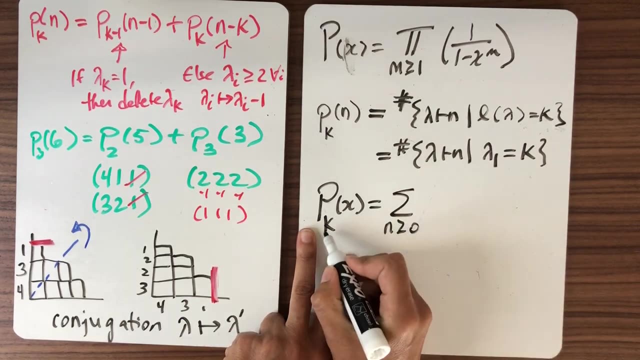 which is the width in this picture, is exactly this operation of conjugation. so they're equi, numerous. and now that we have this, we can reinterpret this formula here. so if I say PK of X, this is going to be the generating function for partitions. now we're fined by K, so this is going to be PK of n- X to the N, if I. 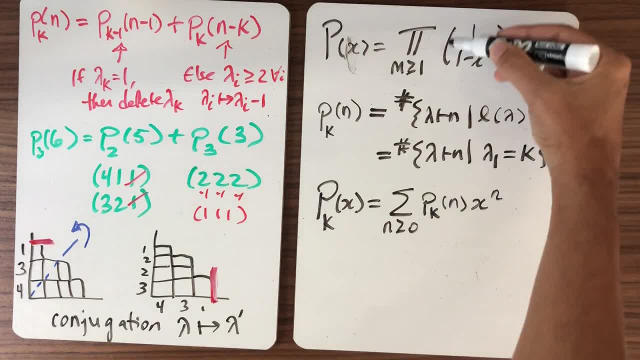 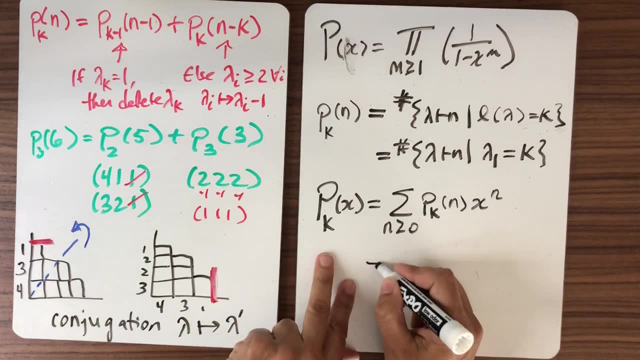 think about what each of these terms means. so choosing an element from this infinite series is telling me how many parts of size M. I've now put a restriction on what M can be, so this is actually a nice thing that we can put onto a computer. this is the product from